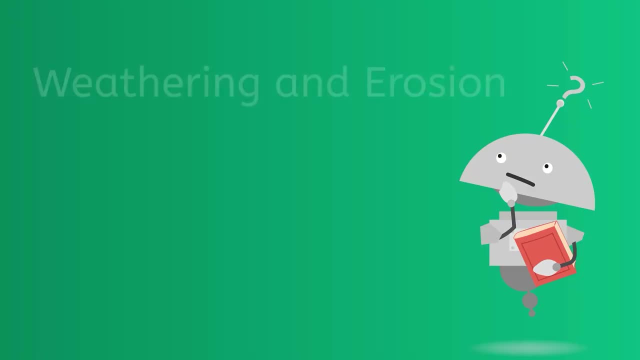 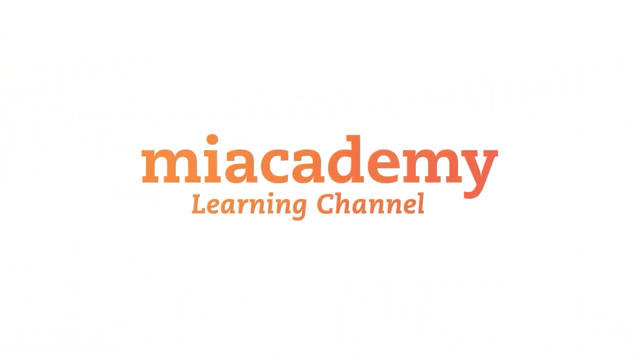 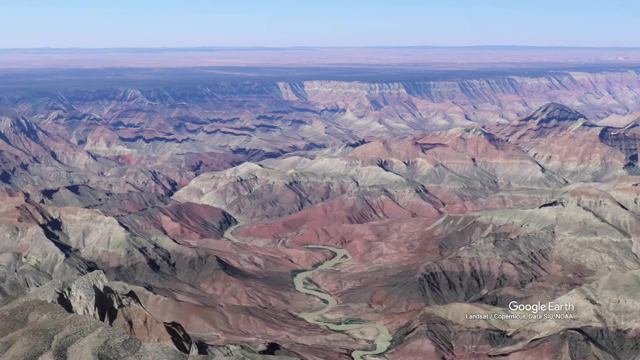 as we explore the powerful forces on the surface of the earth known as weathering and erosion. Let's take a look at the Grand Canyon, arguably the most famous canyon in the world, attracting around 5 million visitors every year and appearing on nearly everyone's list of things. 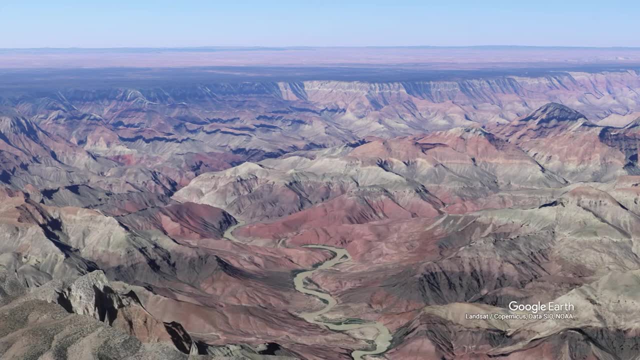 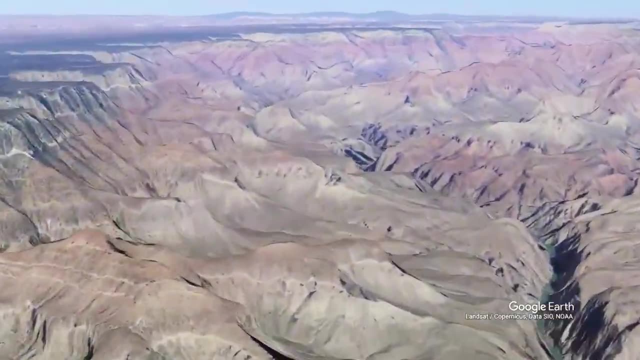 to see before they die. If you haven't seen the Grand Canyon, think of it as a place you haven't seen yet, Because I'd like to think that one day you will, and when you do there's a good chance. you'll agree with explorer John Wesley Powell, who said: the wonders of the Grand Canyon cannot. 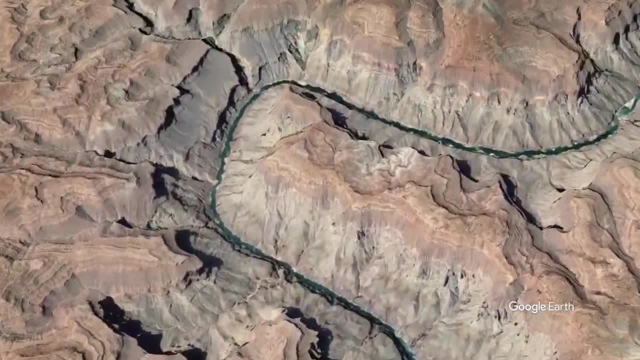 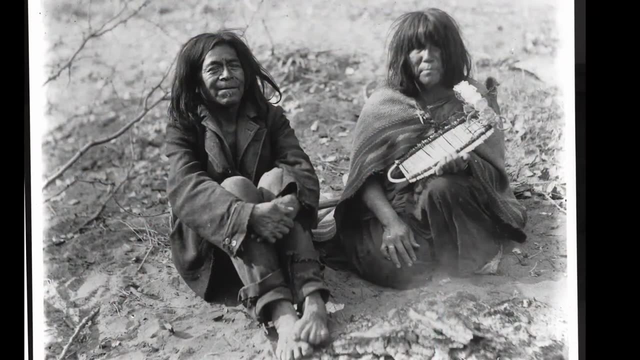 be adequately represented in symbols of speech, not in words. So let's take a look at the Grand Canyon itself. So how did this place that's too wondrous to describe come to be The Havasupai people, who've been living in the Grand Canyon for more than 800 years? 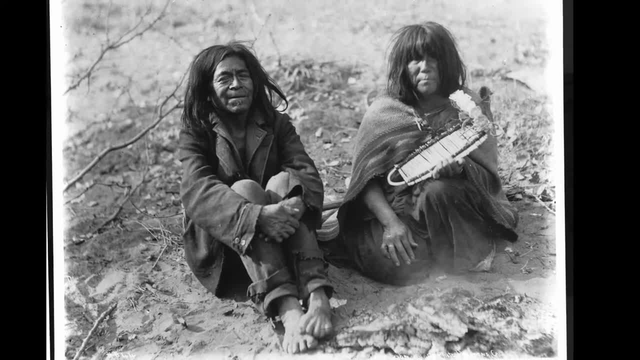 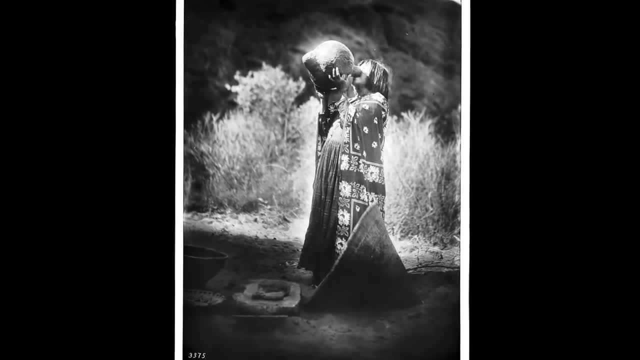 tell a story that explains both the creation of the Grand Canyon and the origin of their people. It goes like this: There were two gods, one of goodness and one of evil. The god of goodness had a daughter. he hoped would be the mother of all living things. The god of evil didn't want. 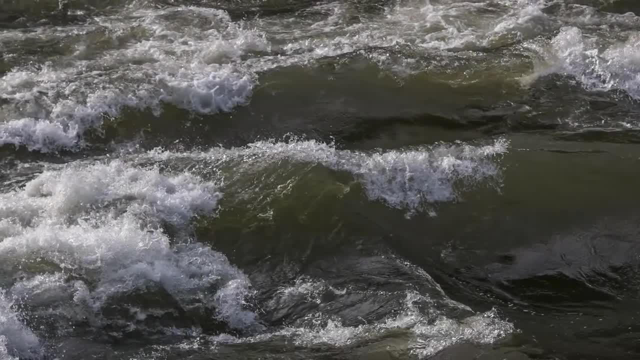 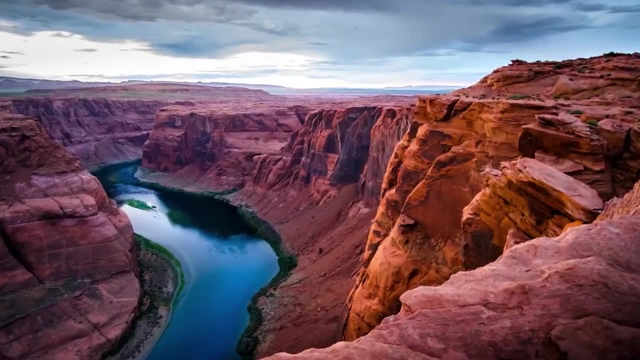 that to happen, so he flooded the world. The good god made a boat from a hollow tree and placed his daughter in it to save her. When the father of the good god, the god of evil, was born, the flood finally receded. mountains rose up and rivers appeared, one of which cut through the. 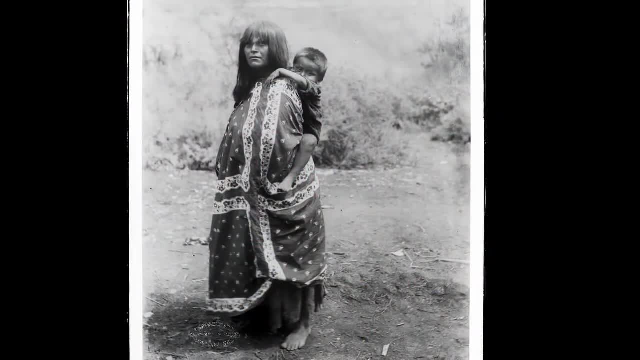 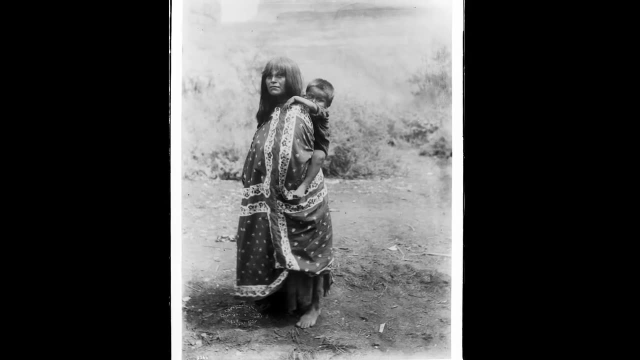 mountains and created the Grand Canyon. When the land dried, the daughter set foot on a new empty earth. Then the sun rose up and caused her to conceive. Soon she gave birth to a baby boy. Later, a waterfall caused her to conceive again and she gave birth to a baby girl. 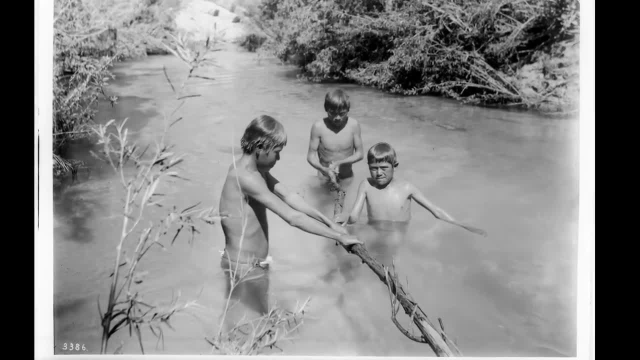 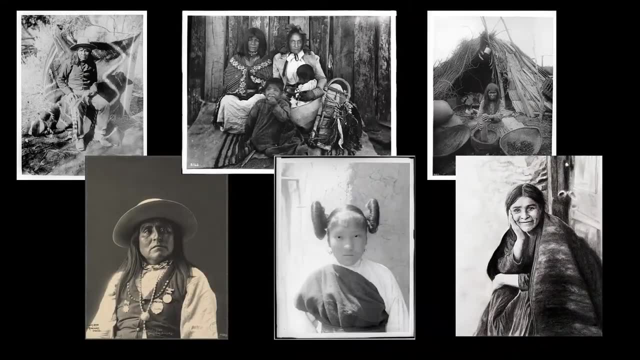 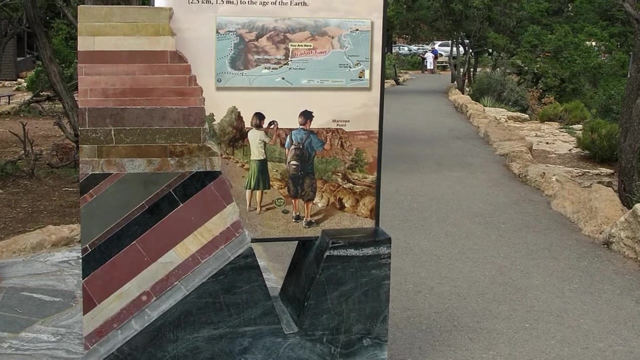 From the union of these two children came all the people on earth. The first of these people were the Havasupai, then the Apache, Hualapai, Hopi, Paiute and Navajo. Now, a geologist telling the origin story of the Grand Canyon might say it began two billion years. 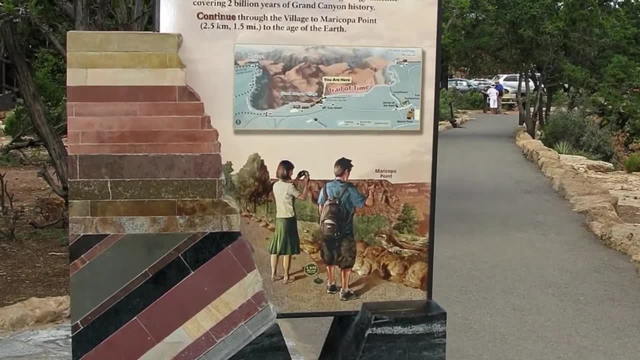 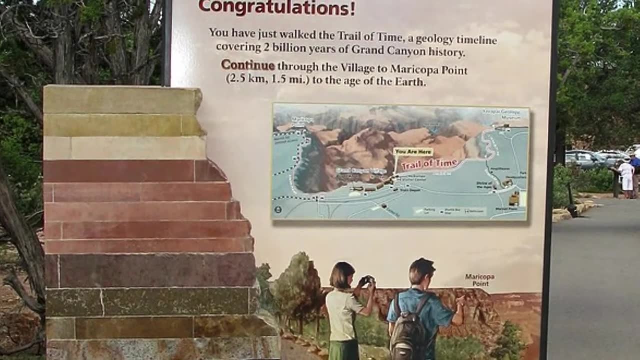 ago, with the formation of igneous rock, which is rock formed within the earth from cooled and crystallized magma, plus metamorphic rock, which is rock that's changed from its original state due to high heat and pressure, along with a top layer of sedimentary rock, which is rock composed. 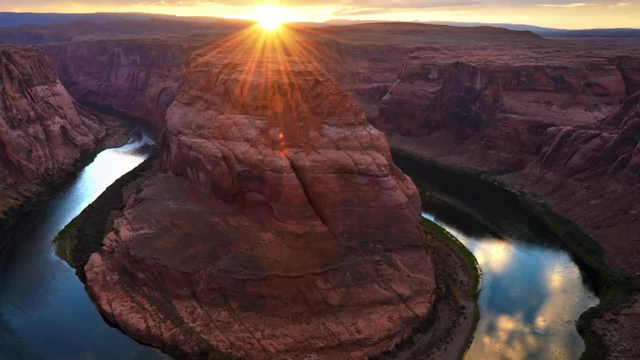 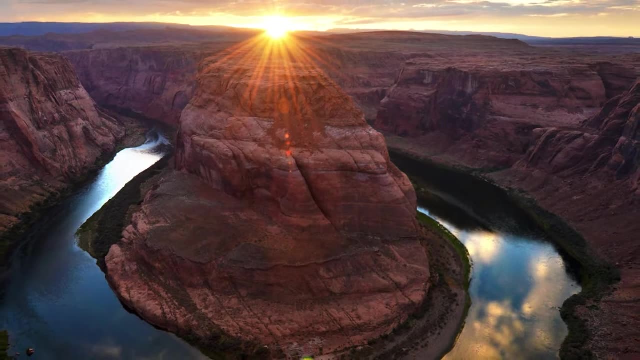 of many smaller rocks formed near the earth's surface. Then, between 70 and 30 million years ago, the action of plate tectonics was made. The rock was then formed into a rock that was uplifted the region and created the Colorado Plateau. Finally, between 5 and 6 million years, 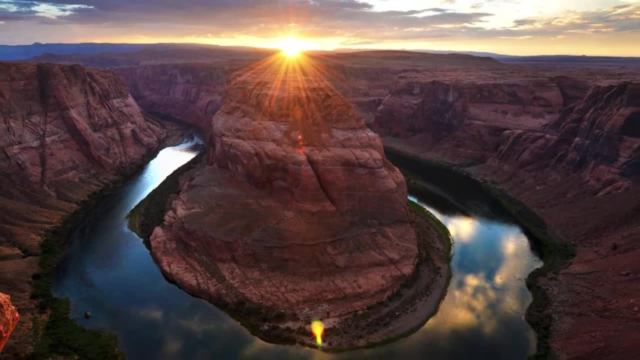 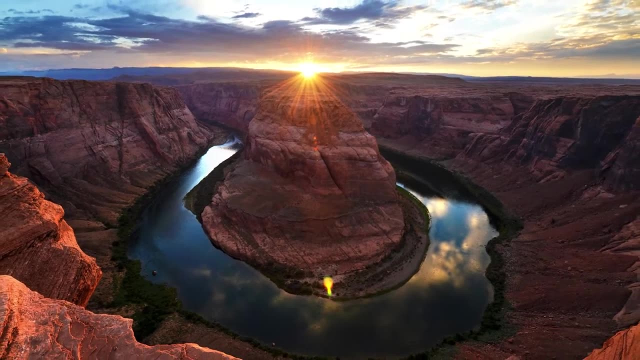 ago, the Colorado River and its tributaries carved and widened the canyon through the powerful processes of weathering and erosion, which we'll talk about in a moment, and which revealed the spectacular layers of igneous, metamorphic and sedimentary rock that we know today as the Grand 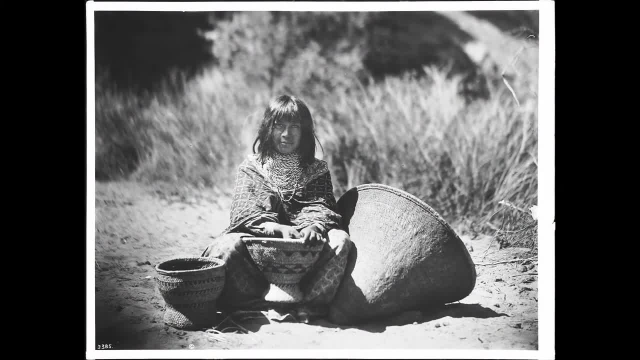 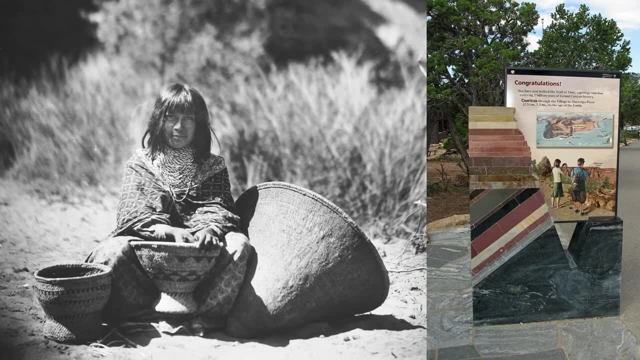 Canyon From a geographic point of view. both the Havasupai explanation and the modern geological explanation have value because both help us understand the truth of the Grand Canyon. Geographers are interested in what people in a particular area think and believe about where. 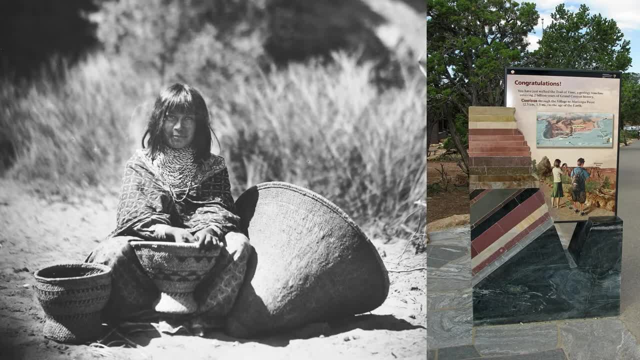 they live about the origins of their place and about the process by which it became what it is today, And this includes myths, legends, history, science, art, literature and everything else that makes up a place's culture. An astute geographer, for example, might notice similarities between the. 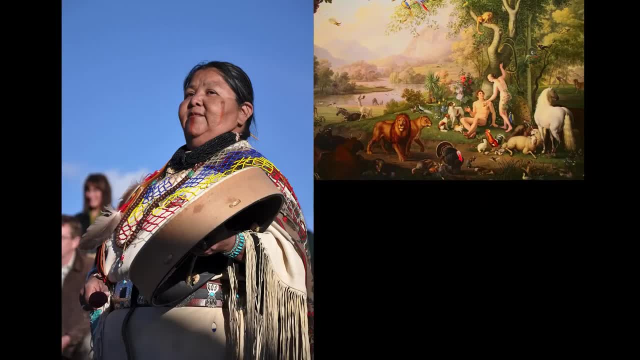 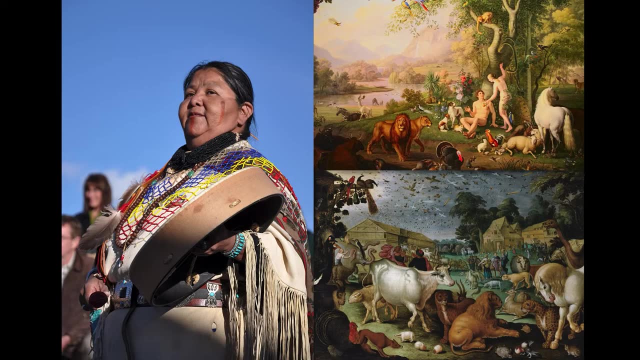 Havasupai story and the biblical stories of Adam and Eve and Noah's Ark, and might therefore consider investigating the possibility of cross-cultural influence between Judeo-Christian tradition and Native American tradition. An astute geographer would certainly notice that both the 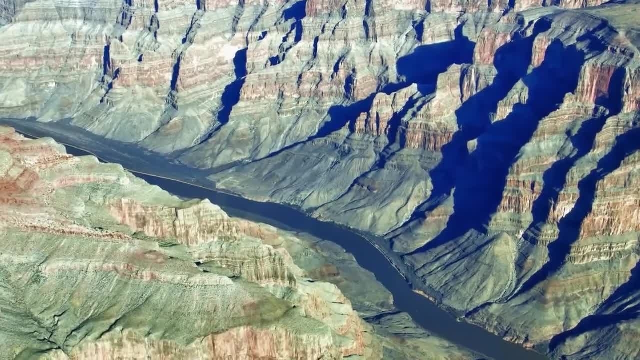 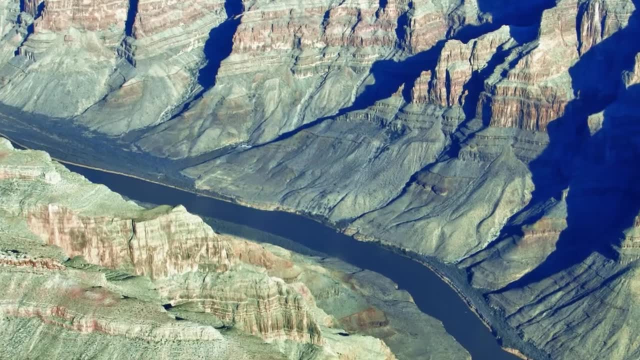 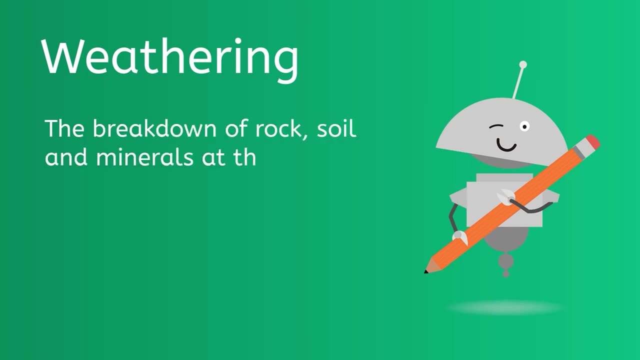 Havasupai explanation and the modern geological explanation involve the process of water carving the Grand Canyon out of the surrounding rock. Both stories point to the actions we know today as weathering and erosion. Weathering is the breakdown of rock, soil and minerals at the 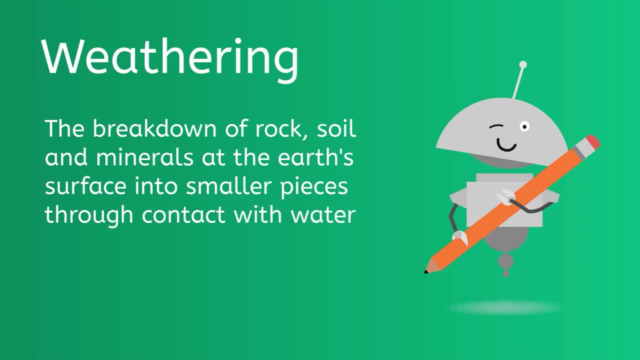 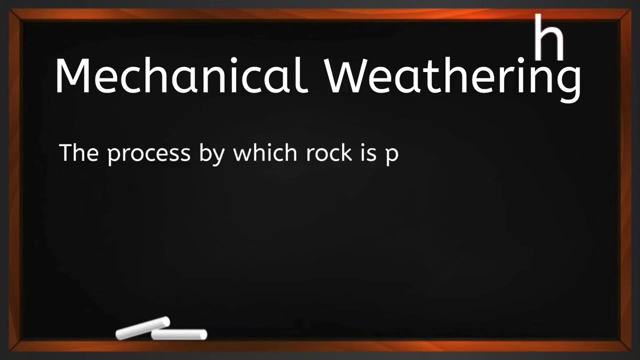 earth's surface into smaller pieces through weathering and erosion. Through contact with water, air and biological organisms, the process of weathering over millions of years can reduce a mountain to pebbles. Geologists identify two kinds of weathering: mechanical and chemical. Mechanical weathering is the process by which rock is physically broken. 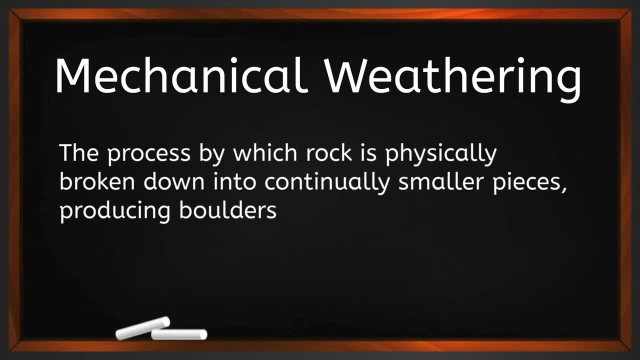 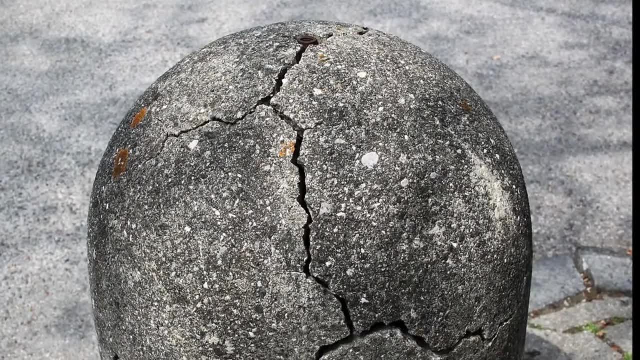 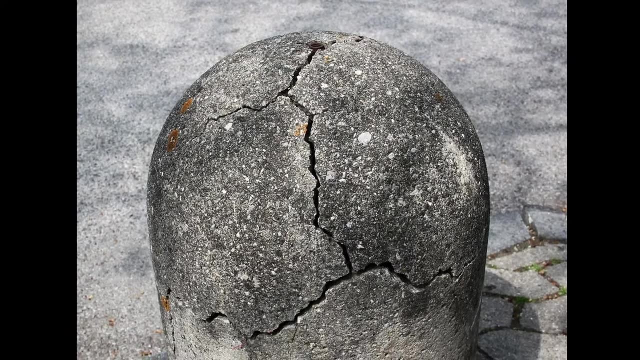 down into continually smaller pieces, producing boulders, stones, pebbles, sand, dust and so on, ultimately building the soil in a particular area. Frost wedging is a common example of mechanical weathering. When water freezes into ice and rock crevices and then expands, the crack widens and over time, 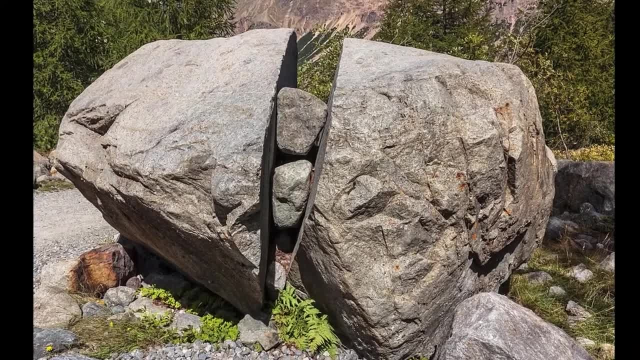 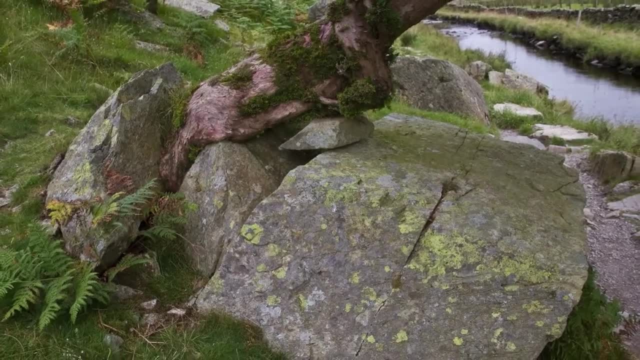 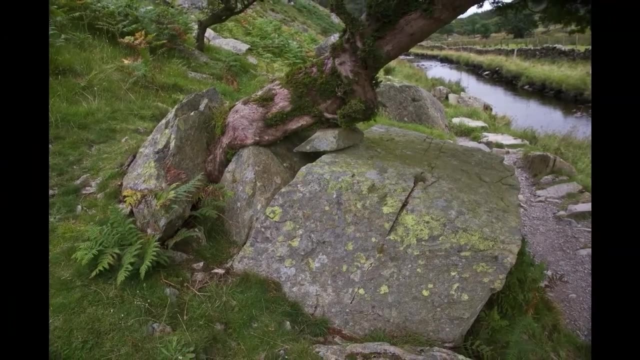 splits the rock. Frost wedging can cause enormous parts of mountains to eventually break and fall away. Other examples of mechanical weathering include tree roots growing in similar cracks, rocks cracking due to forest fires, and rocks expanding and contracting in areas with extreme high and low temperatures. Although mechanical weathering breaks down rocks, it leaves their 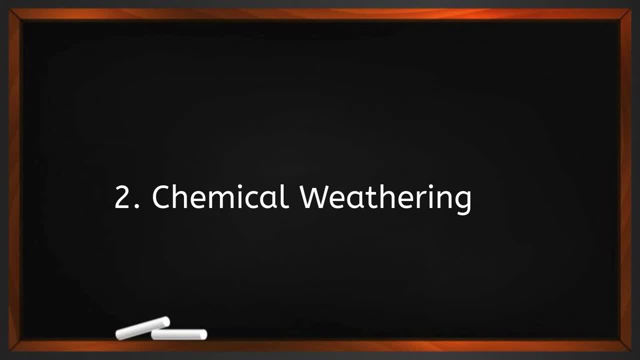 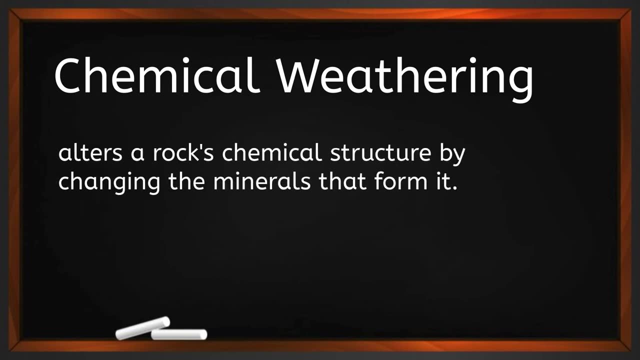 chemical structure unchanged. This is not the case, but it is a common practice. in the case with chemical weathering, which alters a rock's chemical structure by changing the minerals that form the rock, This kind of weathering can actually change one kind of 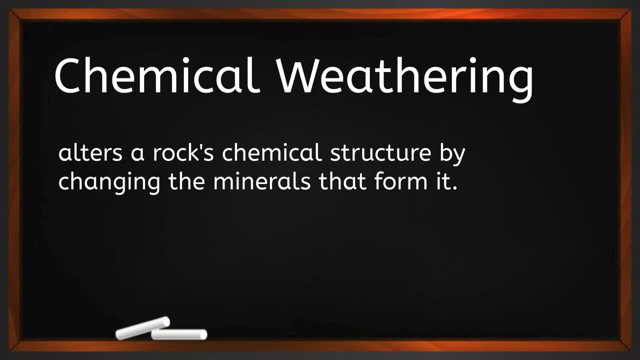 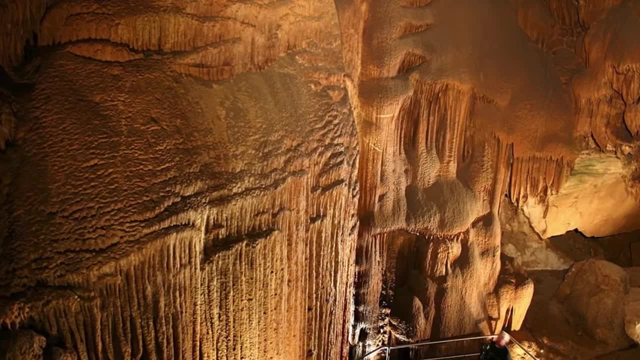 rock into a completely different kind. Sometimes it can dissolve rock altogether, as it did at Mammoth Cave, Kentucky. At Mammoth Cave, carbon dioxide from soil and air combined with water to make carbonic acid, which dissolved large portions of limestone on the earth's surface. 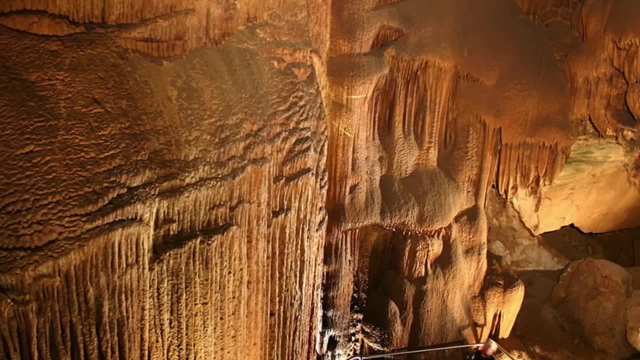 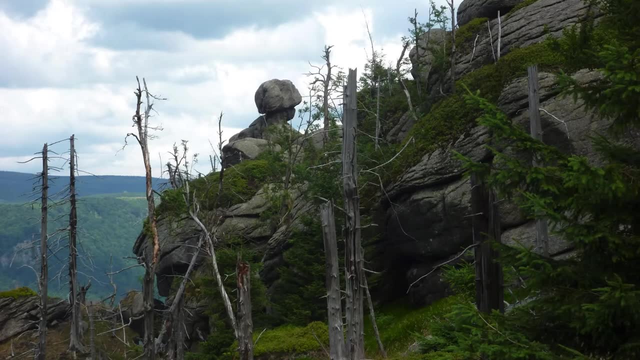 and formed a massive cave system over 405 miles long- the world's longest. Another example of chemical weathering, this one producing very different results, is acid rain, which destroys forests, pollutes water and eats away the surfaces of stone structures and rock formations. It occurs when chemicals produced by industrial pollution or 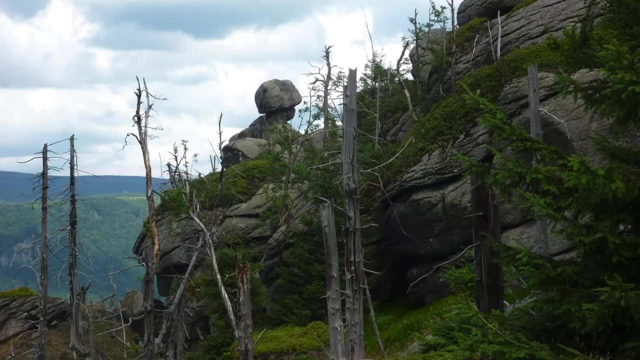 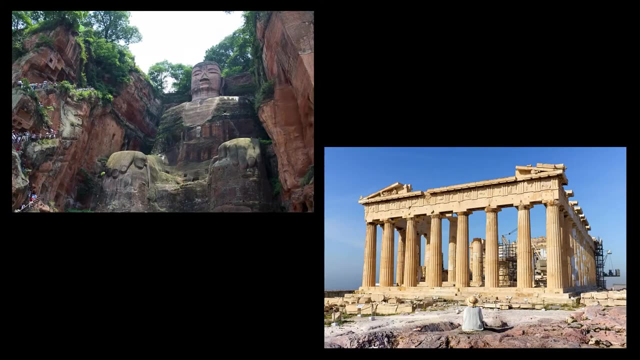 volcanic activity, mix with water vapor and fall back to earth. The Leshan Buddha in China and the Acropolis in Athens are just two of the many World Heritage Sites endangered by acid rain Erosion, the primary force that formed the Grand Canyon. 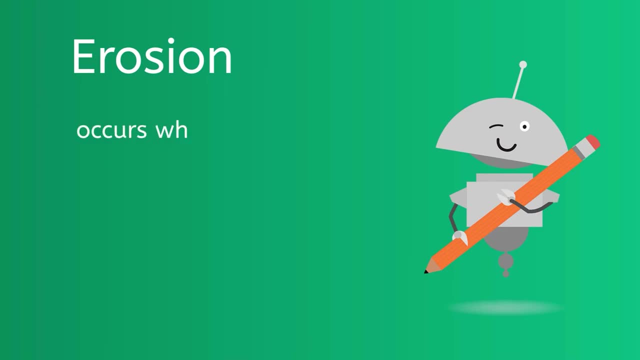 works in a very different way. It's a very different way of working. It's a very different way of working. It's hand-in-hand with weathering. Erosion occurs when water, wind or glaciers move weathered material such as gravel, soil and sand. Erosion is critical to life on earth because it 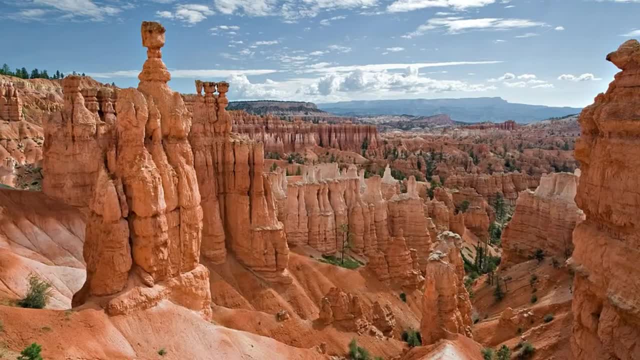 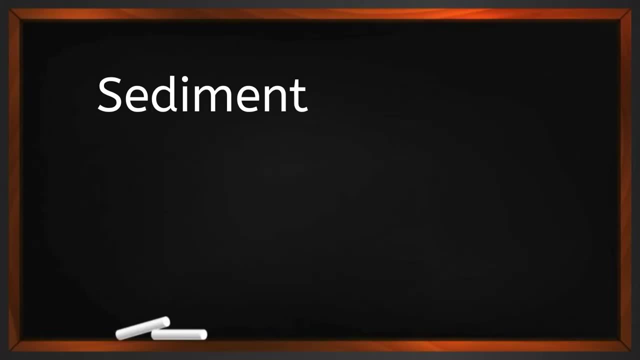 builds the soil that plants need to take root and grow. The largest canyons and valleys on earth were formed by moving water that, over time, cut into rock and wore it away. Water also carries sediment, small particles of soil, sand and gravel that helps grind away at the surface of 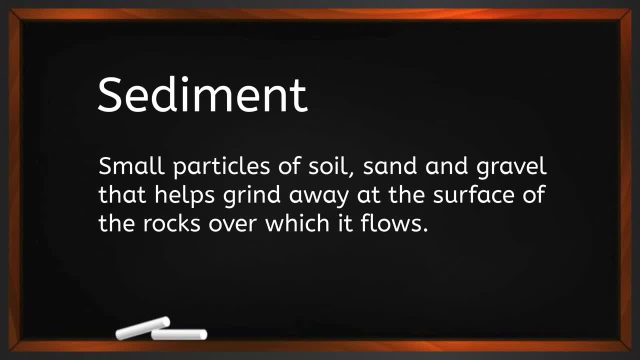 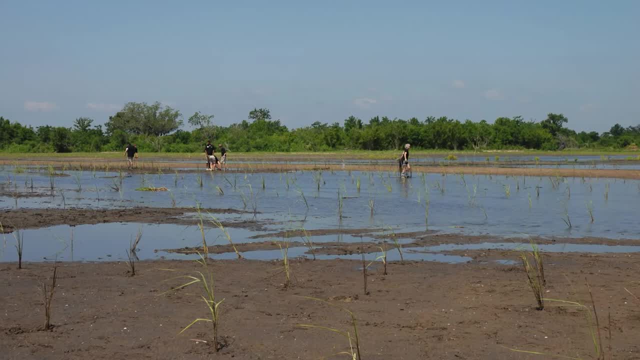 the rocks over which it flows. When the river or stream of water is cut into rock, it's a great source of sediment. When the stream slows down, the sediment piles up and creates new land forms. A broad flood plain or alluvial plain might form on either side of the water, or a low-lying 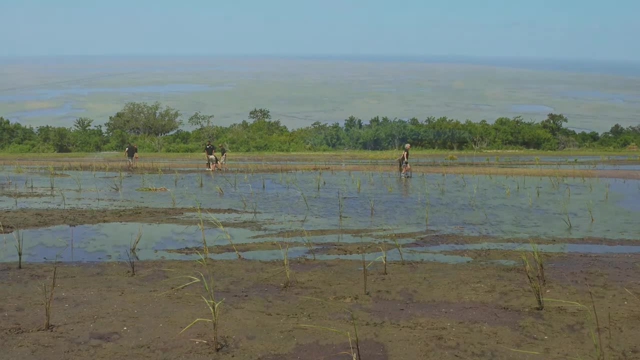 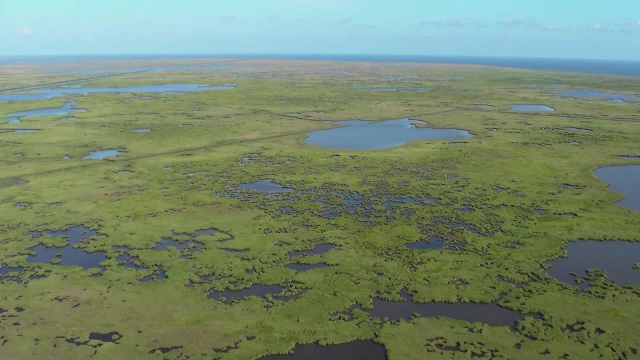 plain, known as a delta, might form where the river enters a lake or the ocean. The Mississippi River, for example, deposits millions of tons of sediment each year along its enormous flood plain and in its delta, where it empties into the Gulf of Mexico. Wind is also a powerful agent of erosion. 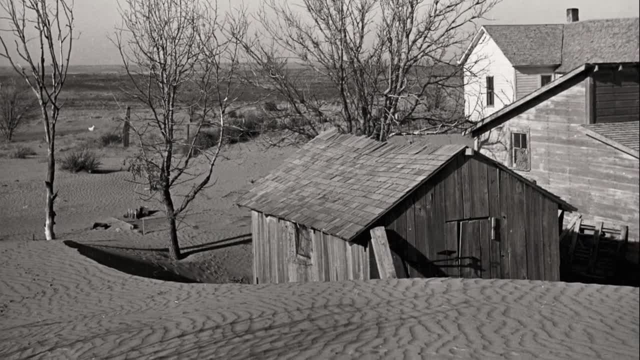 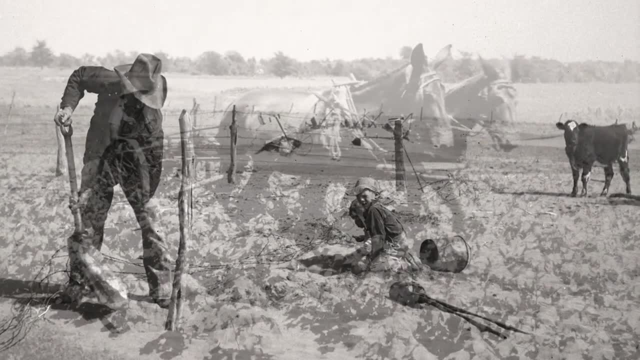 particularly in areas with little water and few plants, making it a great source of sediment. Wind erosion devastated the Great Plains during the Dust Bowl of the 1930s, As the population grew and more land was plowed under huge swathes of. 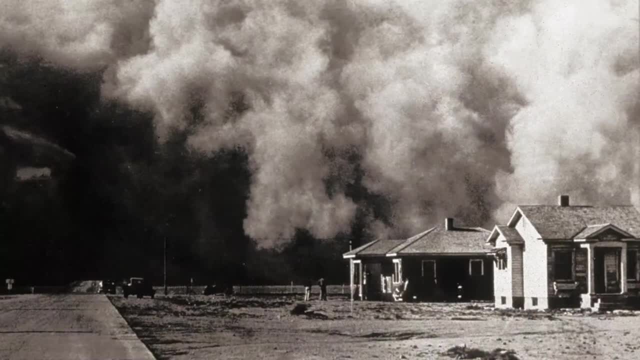 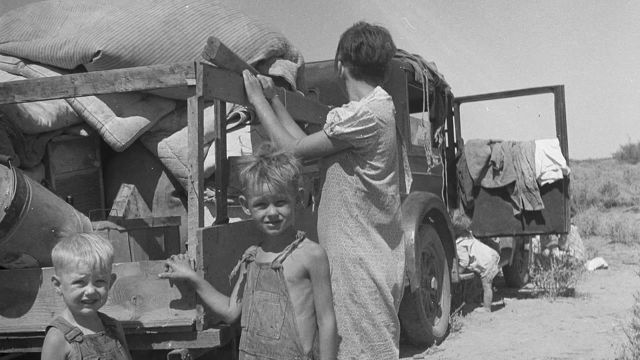 land without plant life were left exposed to the wind, which carried away the topsoil in huge dust storms, leaving thousands of American families with no food, no livelihood and no choice but to migrate west to greener pastures. John Steinbeck's prize-winning novel The Grapes of 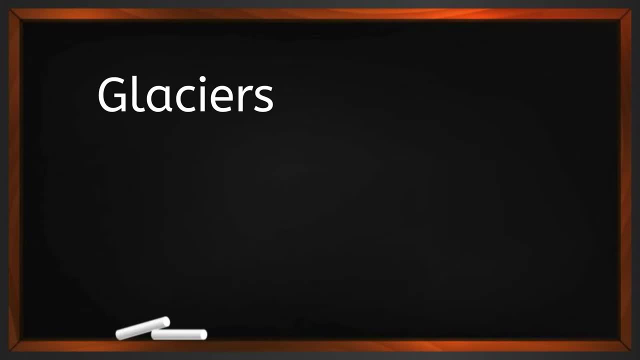 Wrath centered on the struggles of one such family. We mentioned glaciers earlier, but they're worth mentioning again. The Grapes of Wrath are a great source of sediment and they're a great source of water. Glaciers are huge, slow-moving sheets of ice containing dirt, rocks and boulders. 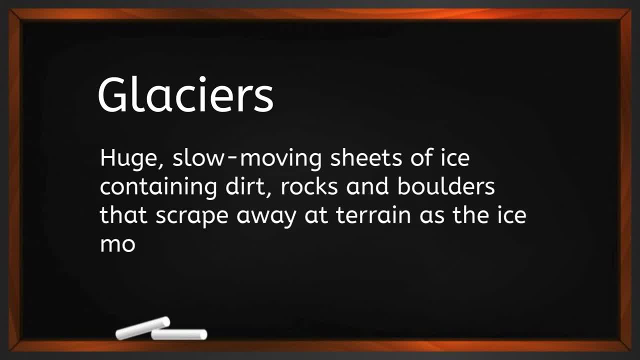 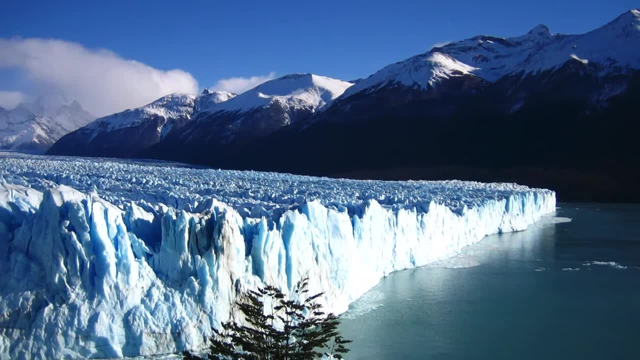 that scrape away at terrain as the ice moves over it. During ice ages, when the Earth's temperature was much colder than it is now, much of the Earth's water was frozen in massive glaciers that covered a third of the Earth. Glaciers carved out the Great Lakes and other smaller lakes in the 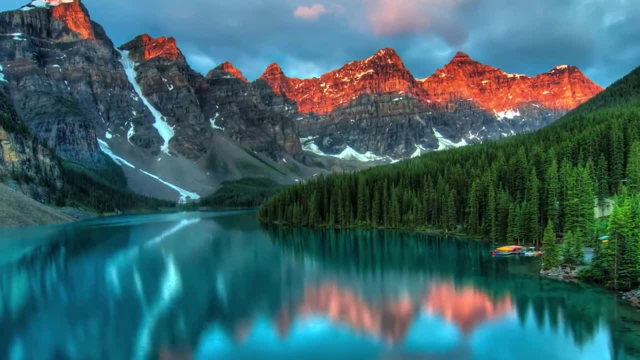 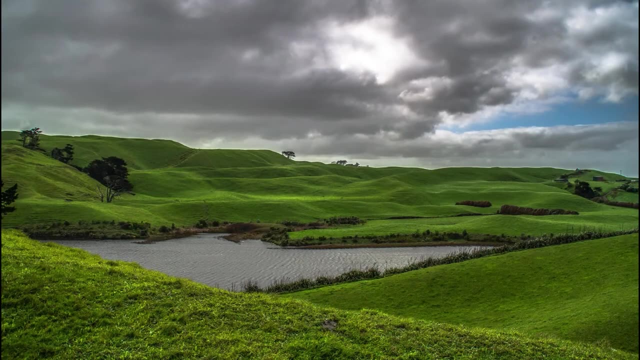 northern part of the United States and when they melted and receded, left behind piles of ridge-like debris called moraines. Some 50 million years ago, there was a landscape of water that was rolling hills and meandering streams in what is now central California. After a series of 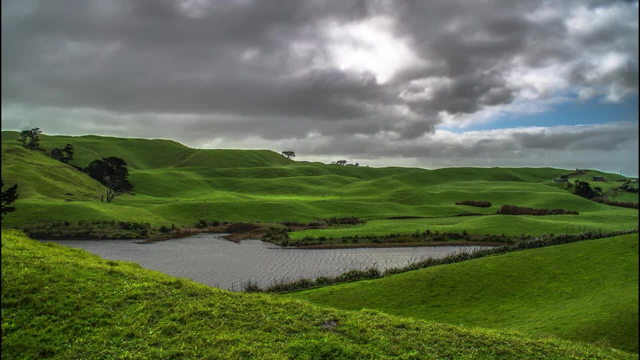 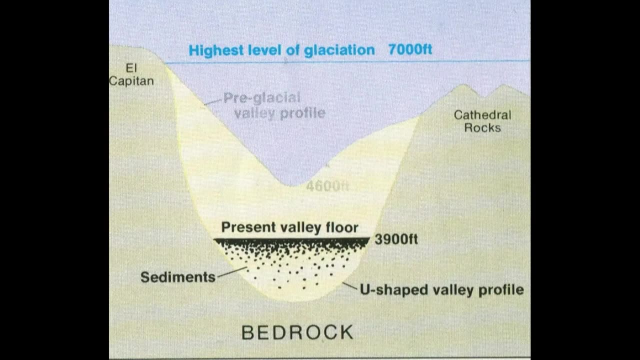 tectonic uplifts and the creation of a canyon by erosion from the Merced River. the canyon was gouged and quarried into a U-shaped trough by a series of glaciers. When the last glacier melted some 10,000 years ago, a spectacular sight was revealed—Yosemite Valley, one of the most visited. 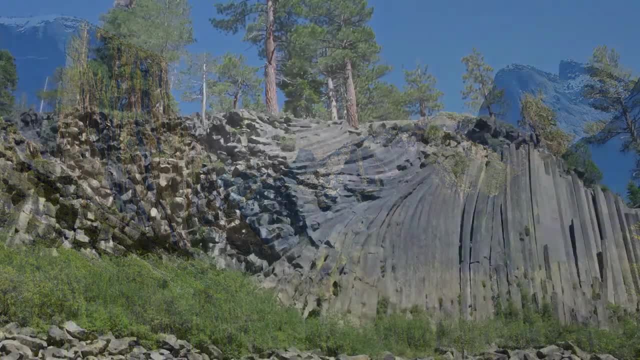 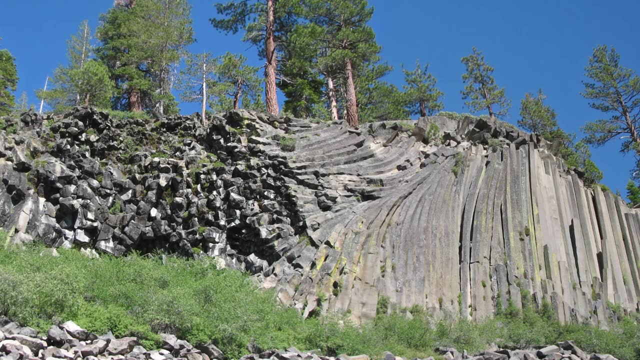 and photographed natural landmarks in the world At Devil's Postpile, only a few miles from Yosemite. hot basalt lava flowing down the Yosemite River was a great source of water for the Yosemite Valley. The Yosemite Valley was met by a receding glacier. Because of its thickness, the lava